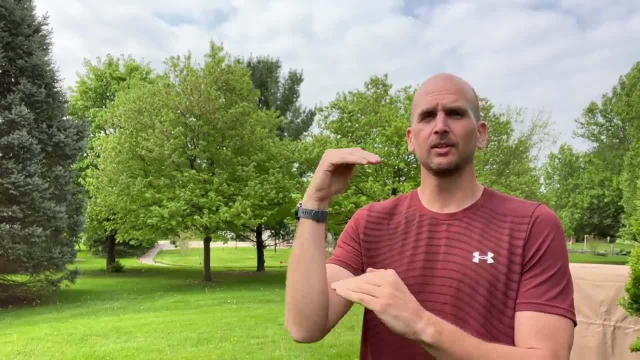 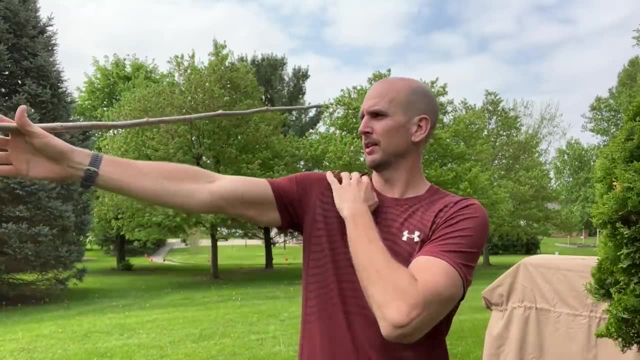 apply it to other things like estimating the height of your gutters off the ground, your roof line or anything else outdoors. So anything you need is a stick, and I would make it a little bit longer than the length of your arm. That's going to be the distance from your eye to where you'll. 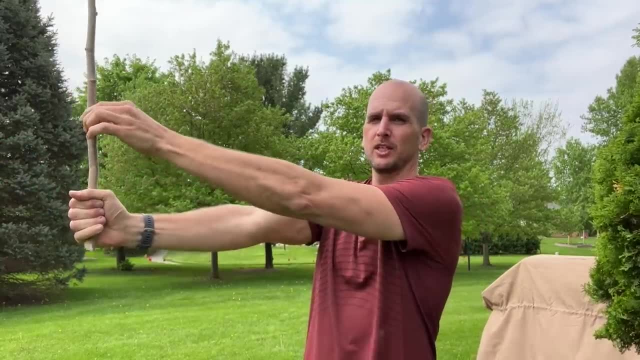 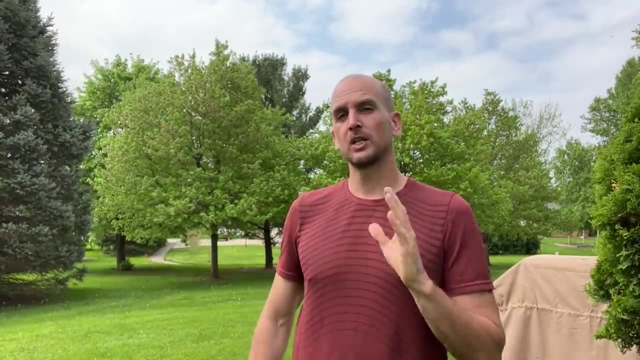 hold it in your hand and if it's a little bit longer, then you can adjust the height slightly, which will match up to make sure that your arm and the stick are exactly the same length, Which helps you get an accurate measurement. So, taking that stick and backing away from the tree, 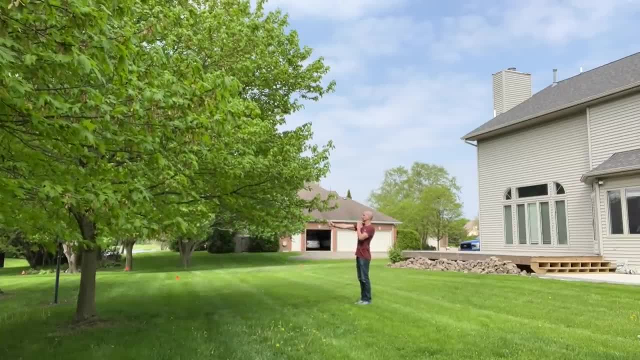 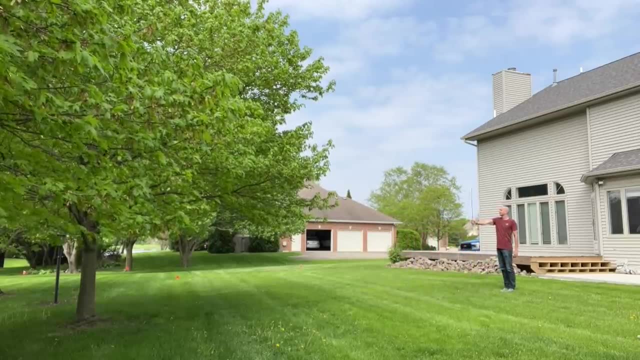 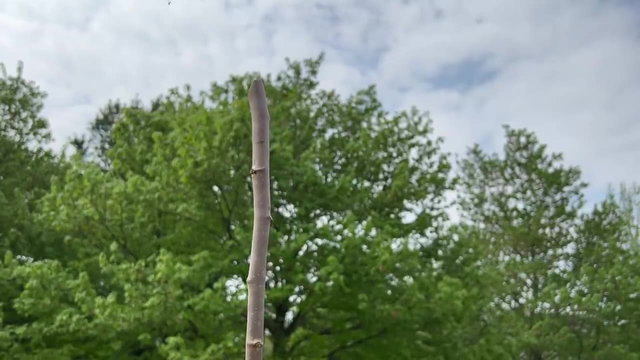 that I want to measure. I'll make sure the stick is the same length of my arm and hold my arm parallel to the ground and the stick perpendicular to my arm, Then backing away and moving towards the tree trunk or away to line up the end of the stick to the top of the tree. Once I get that, 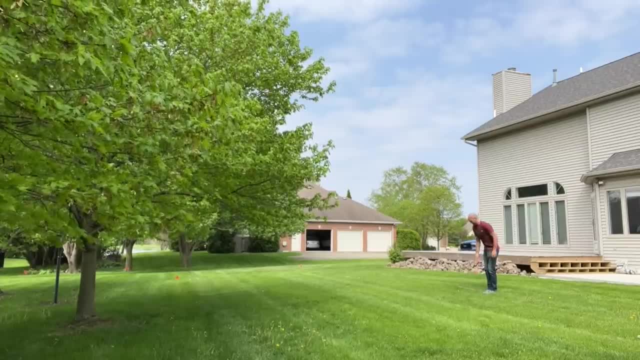 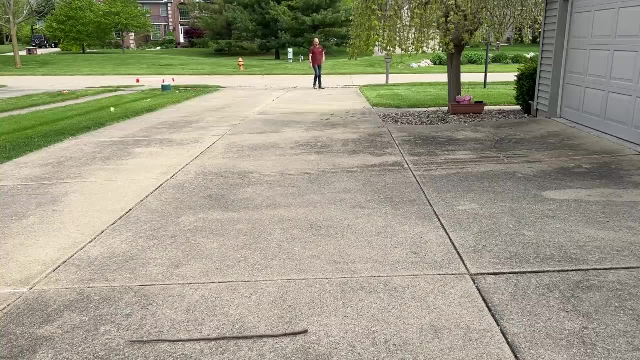 lined up. I can stop, mark the distance away from the trunk and then I'm going to measure the length of my stride length, just to walk off the distance to the tree trunk. If you do not know your stride length, it's easy to get. You can just mark off a standard distance here at 60 feet and 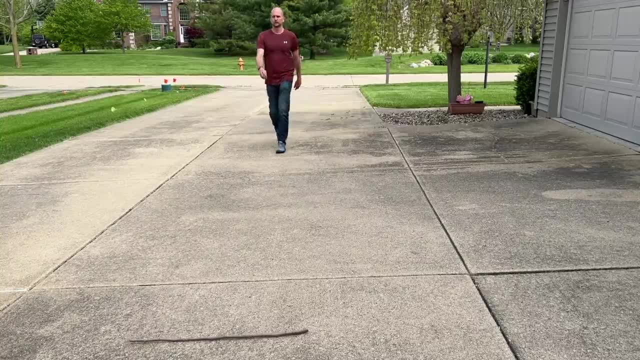 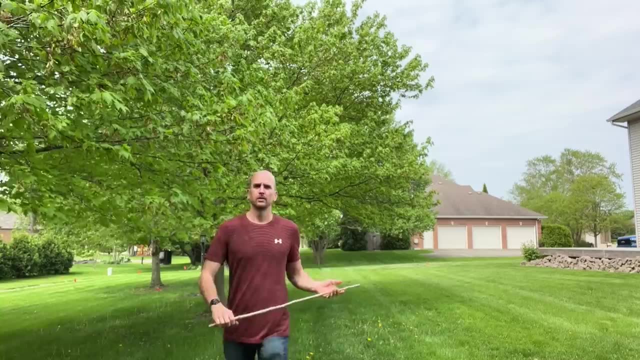 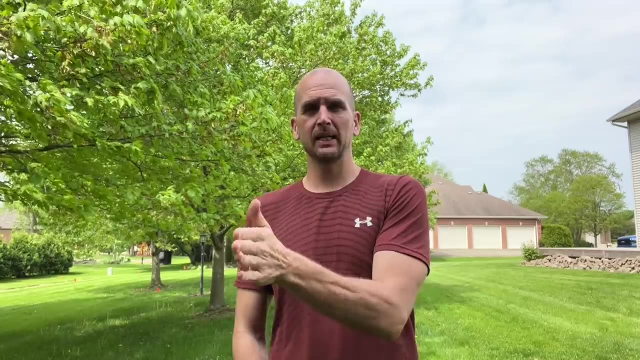 then consistently and comfortably walk or stride that out. and here I will get 19 steps, which gives me about three feet per step or stride. So now I have the information I need to make my estimate. You saw, I took seven steps between where I marked on the ground to the base of the 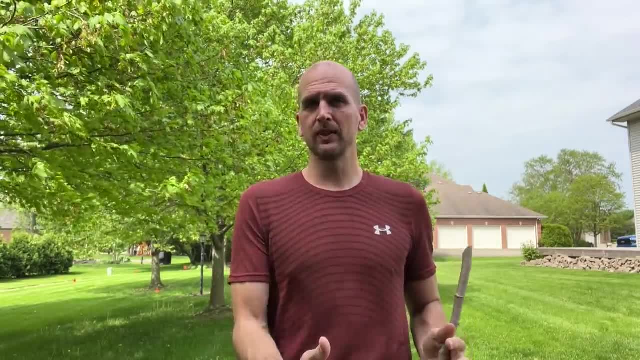 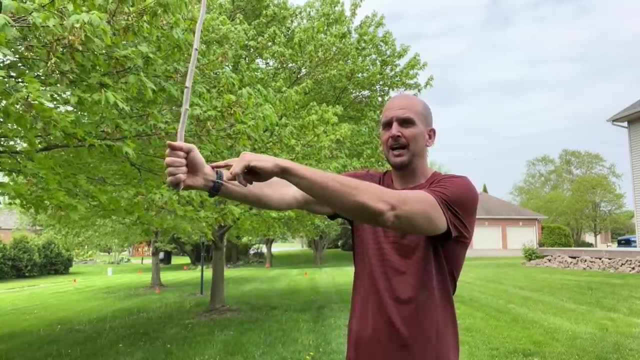 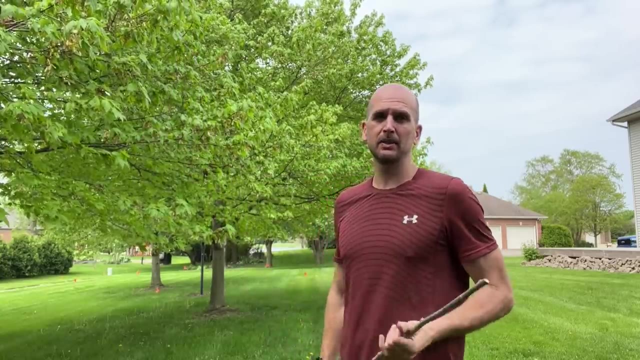 tree trunk. So with my stride length being three feet, I'll multiply that out and get 21 feet. The only thing you don't want to forget is that is actually measuring the height from that arm or your eye level. So for me, I'd want to add five and a half feet, So my estimate is 26 and a half. 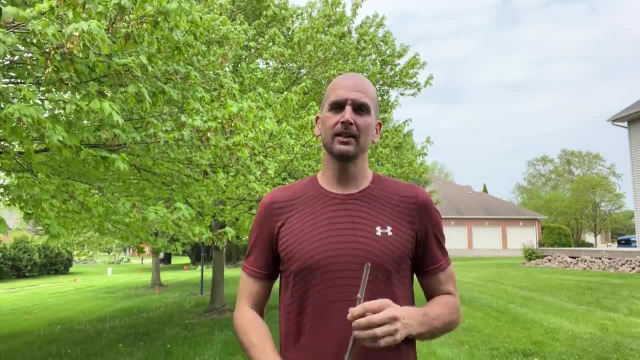 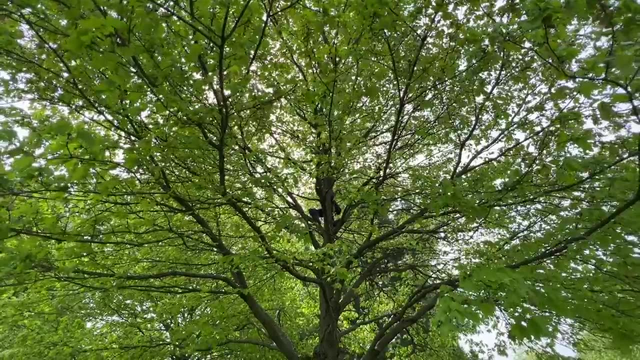 feet is the height of this tree. So let's validate that and see how close I got. Really, this just gives me an excuse to climb trees, which is my favorite pastime. So I get up in the tree and I'm going to measure, just with my normal tape measure, vertically until I get to the top of the 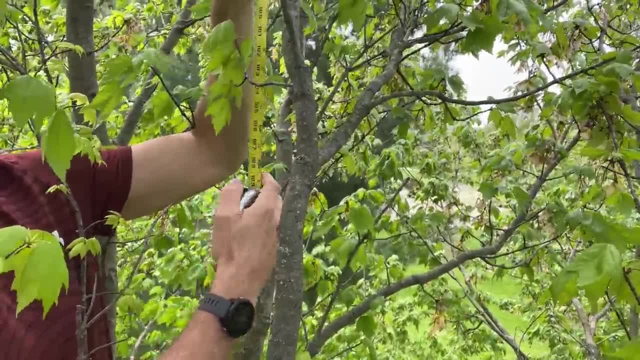 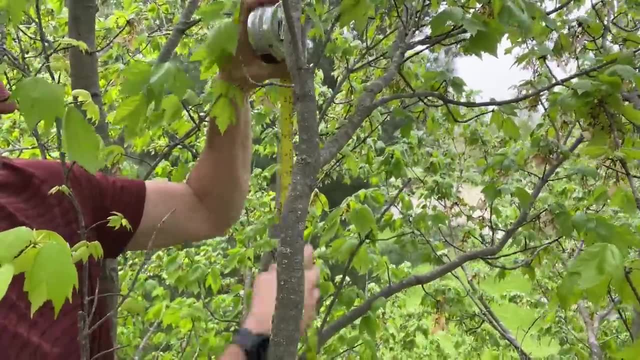 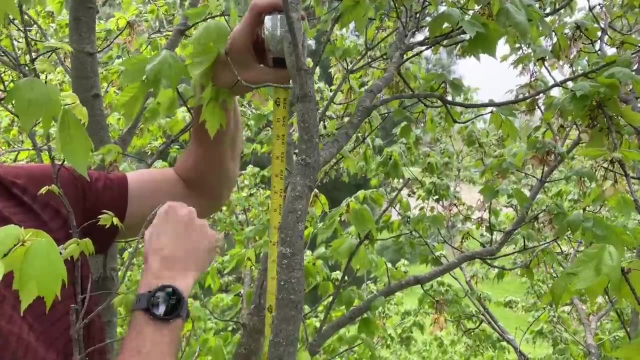 canopy, and in this instance it's going to be right at about nine feet. Then, from that same point, I'll go ahead and measure down to the ground and then just add these two together. So our first measurement was nine feet and now we're looking at about 18.. So just right under 27 feet, Half a foot. 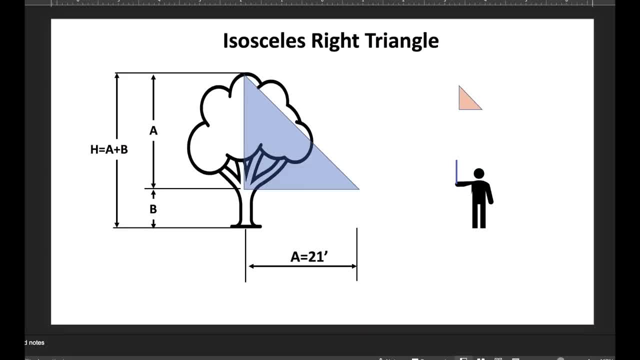 over that distance is about a two percent error, So that's as good as you can really expect. And then the last part is: why? Why does this work? And that goes back to your geometry lessons, which you thought you would never use in school. Well, 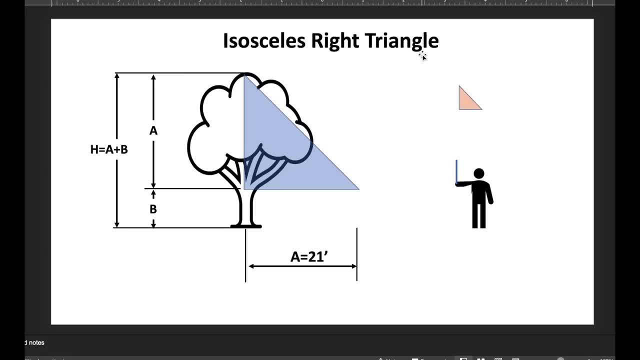 they actually do come in handy and that is the understanding of triangles. So this is a very specific triangle called an isosceles right triangle. We have two sides of the triangle which are the same length, and remember the stick was perpendicular to our arm, which 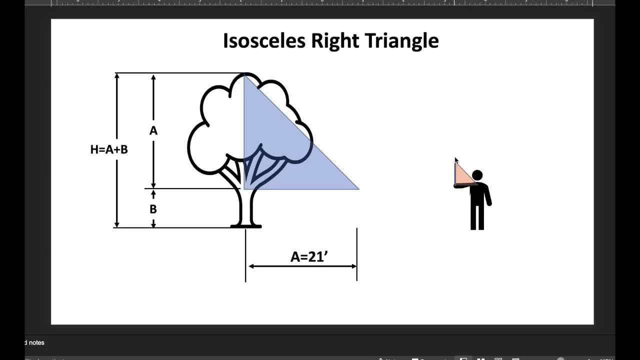 was horizontal to the ground, So we created a small isosceles right triangle. Now how we use this is from our eye, looking past the top of the stick, to the top of the tree, we can align ourself where the distance we are away from the tree perfectly aligns: from our eye to the top of 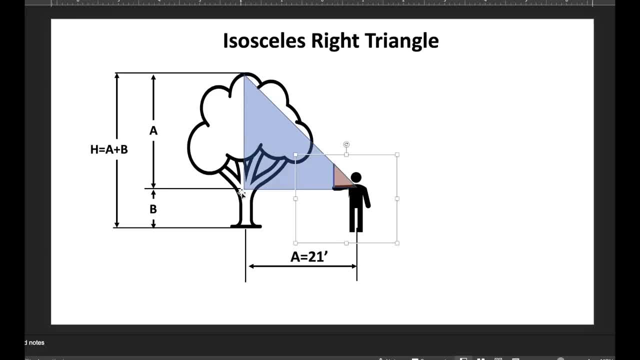 the stick to the top of the tree. So now we have a much larger isosceles right triangle Where we know the side that we are: the distance from the tree trunk to our body. that distance is the same distance from the level of our arm being held out to the top of the tree. So a is equal to 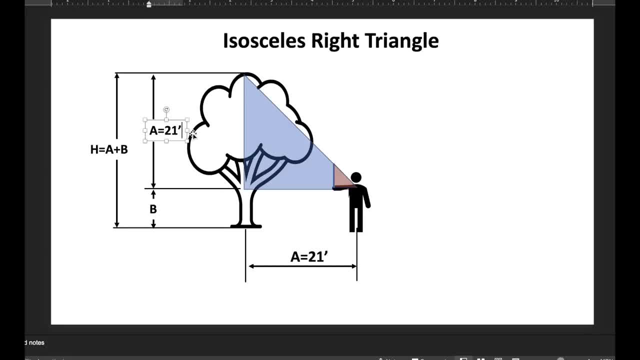 a. So in this case we know that a is 21 feet tall. So to get the height of that tree, once we've lined everything up, all we have to do is add on the distance. our arm is to the top of the tree, So 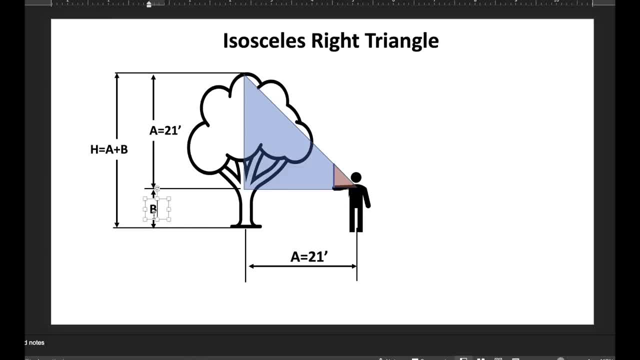 that's our height. Of course, a plus b is equal to a plus b, that's really the height of this tree. So we know that height of this tree is from the ground surface And in my case I said it was five and a 1.5 feet, and you'll just know. in your case you can do a quick measurement to get that. So to